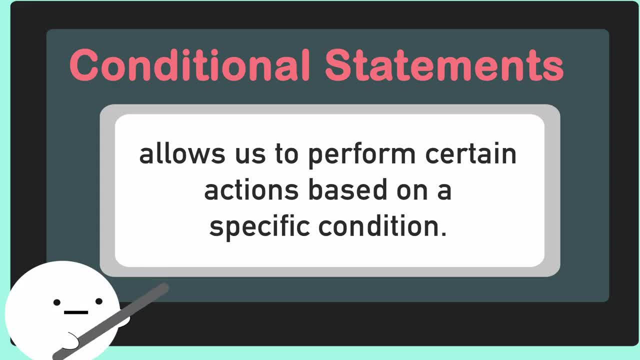 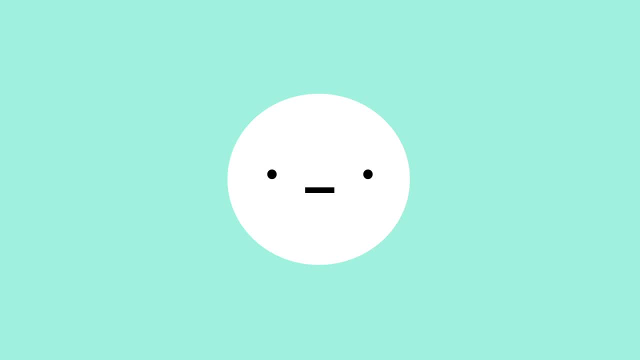 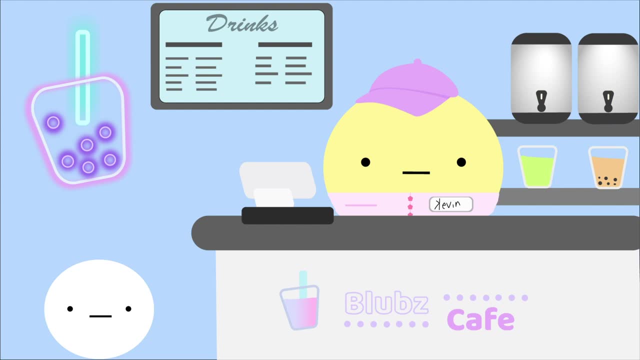 Let's talk about conditional statements. Conditional statements, let us perform actions based on if a condition is met. We use them to help direct the behavior of our programs. In fact, we actually use conditional statements in our everyday lives. Have you ever gone to a cafe but didn't really know what you wanted to order? 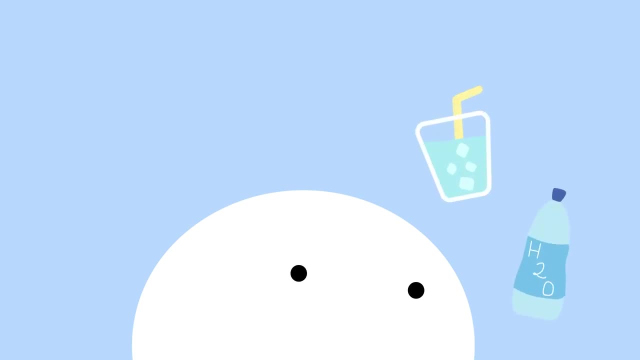 You've probably narrowed down what you want kind of like this: Do I want something refreshing or something thick? If I want something refreshing, I guess I could get something like an iced coffee or an iced tea. I guess I'll get some tea, but what flavor do I want? 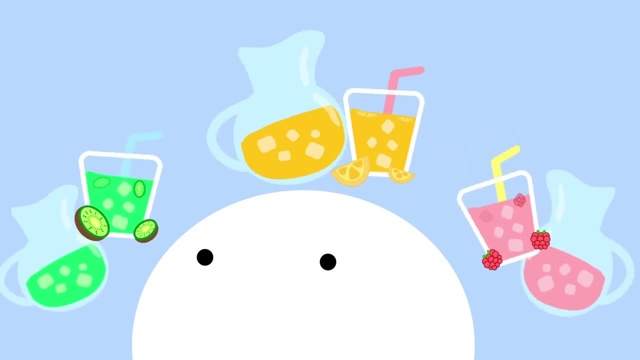 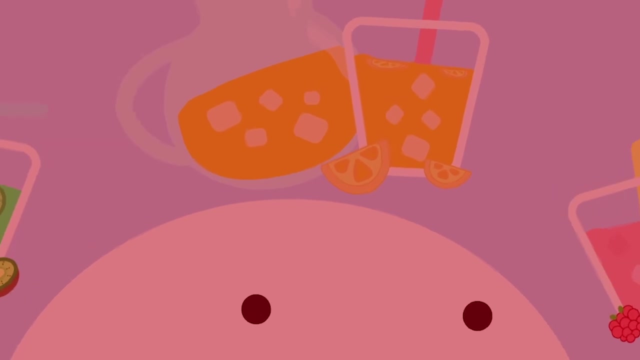 Oh god, there's so many flavors to choose from. Am I feeling a little adventurous? or should I pick something safe, Something tart, Maybe something citrusy, Maybe strawberry? But can I even afford this? What am I doing with my life? Do my parents even love me? 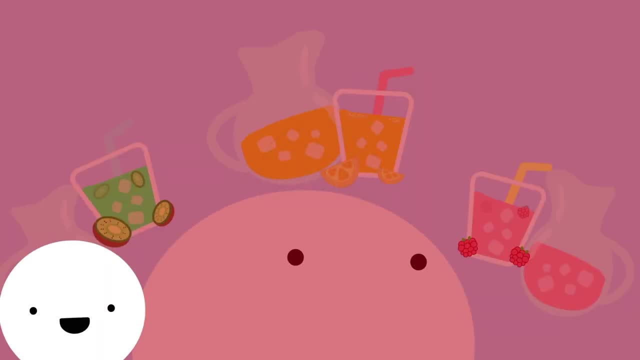 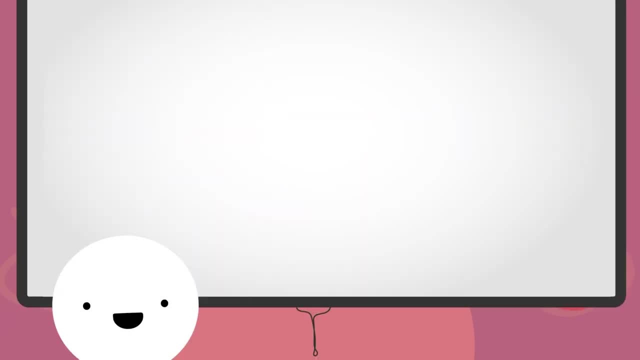 To figure out what we want. we can use something called a flowchart. Flowcharts help us plan and visualize the different outcomes in our program. Looking back at our cafe scene, we can use a flowchart to figure out what we want to get. First we ask ourselves: do we want something? 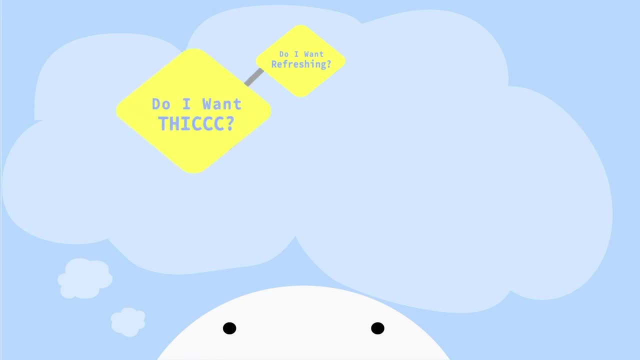 refreshing. If not, do we want something good? If we do, then we'll get a smoothie, But if not, we'll just not get anything at all and go home. But if we choose to get a refreshing drink, then we ask ourselves: do we want tea? And if 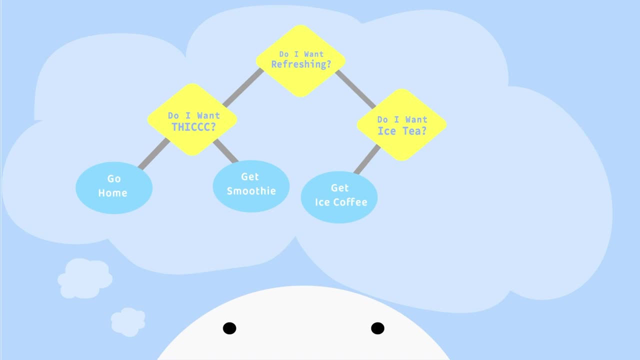 not, then we'll get an iced coffee. But if I do want tea, then do I want raspberry? If we do, then great, we'll get raspberry, But if not, we'll just get some kiwi flavored tea instead. 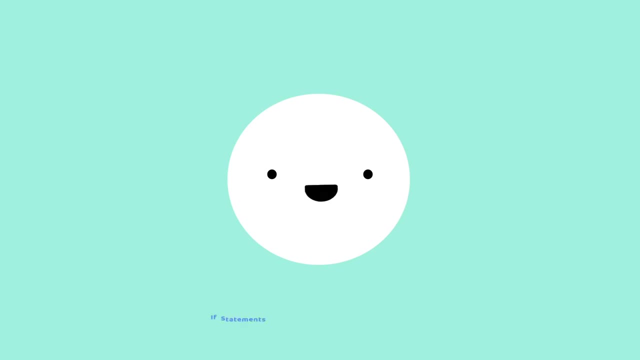 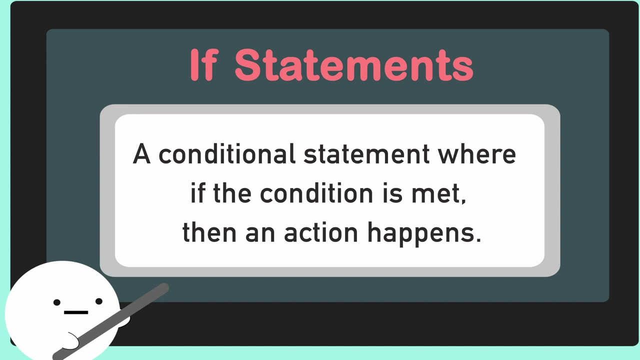 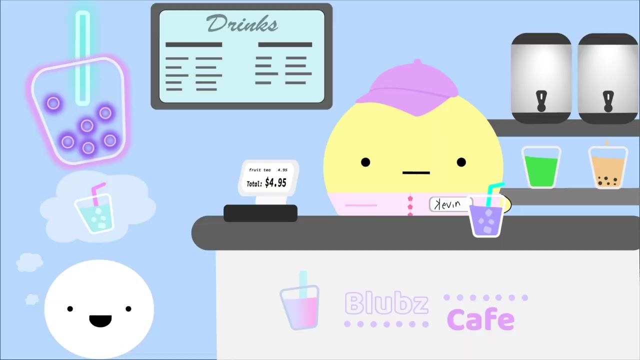 In programming you can represent these decisions with what's known as an if statement. An if statement is a conditional statement where if the condition is met, then an action happens. So if I'm in the mood for something refreshing then I'll order a fruity drink. Now that we have an. 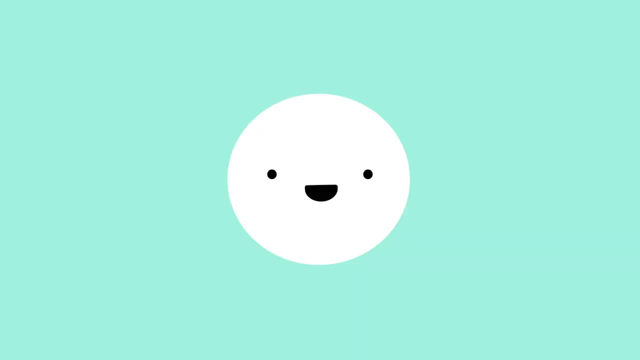 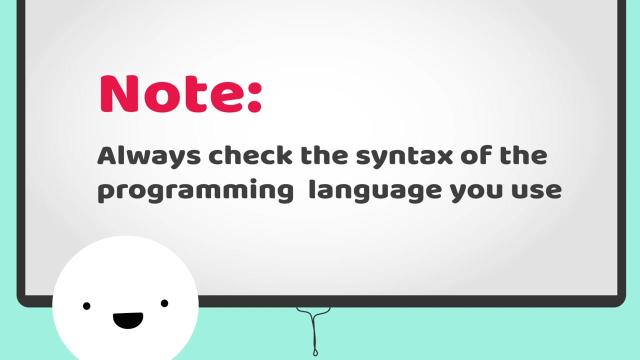 idea of what an if statement is. let's see how we go about writing one. As a disclaimer, even though writing an if statement is pretty much the same in most modern languages, it's important to check your specific language to make sure you didn't miss. 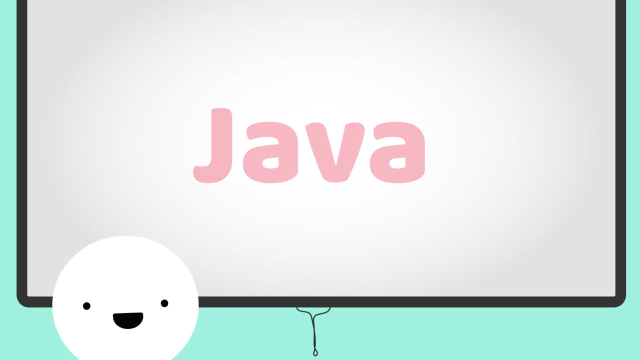 anything. In this case we're using the language Java, But this would also work for the languages C, C++, C, Sharp and JavaScript. Anyways, back to the video. We start an if statement by simply putting the word if at the beginning of two parentheses. Then 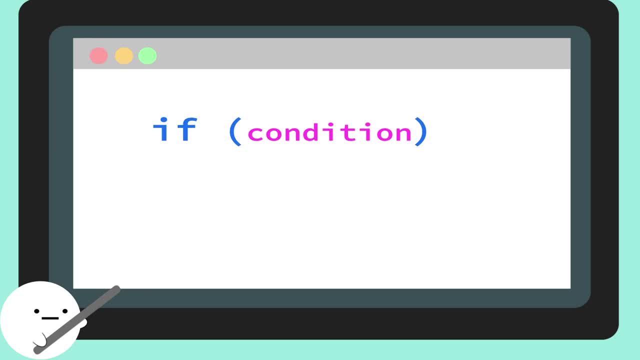 you would follow along with the following sentence: If you have an idea of what an if statement is, you can follow up with a condition. A condition is something that we check to see if it's true, And if it is, the computer will execute whatever's inside our little curly brackets. 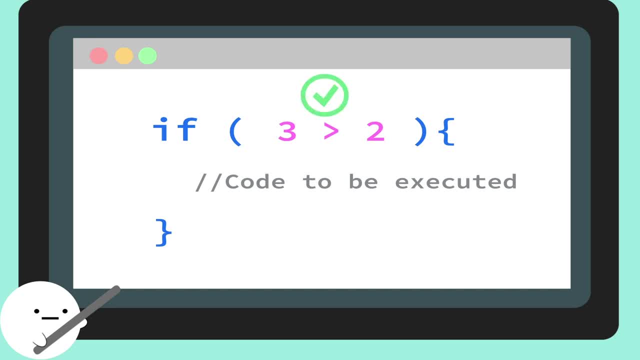 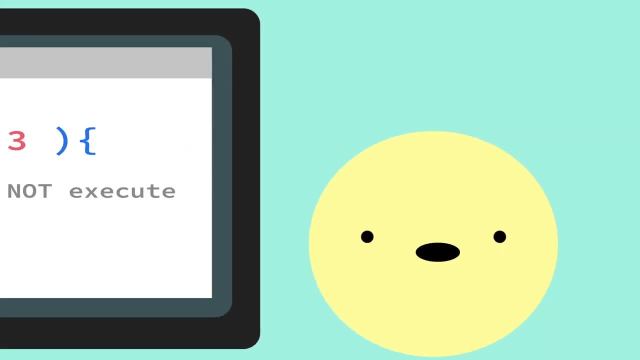 Like: is 3 greater than 2? It is, So it'll execute the code, And if it's not true, then the computer will just continue reading through your code and ignore whatever you wrote here between the brackets. Voila, What are some ways we can check our condition? 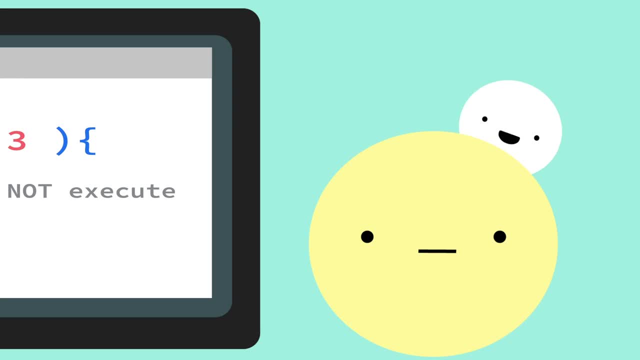 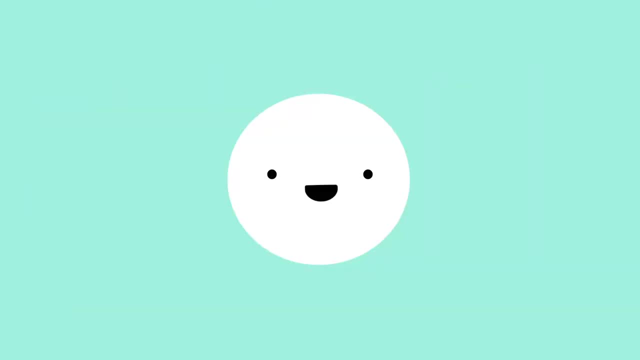 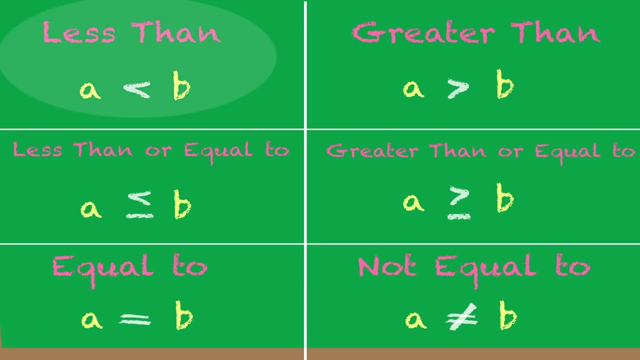 I'm glad you asked, Kevin. The way we check to see if our condition is true is by using comparison operators. These comparison operators are exactly what you'd see in your elementary class: Sit down and shut up. We got the less than, the greater than and well, you know the rest. 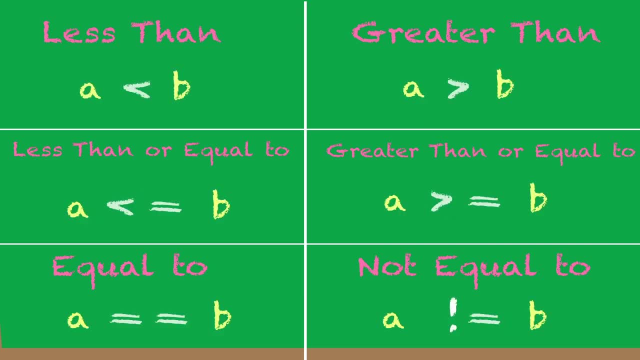 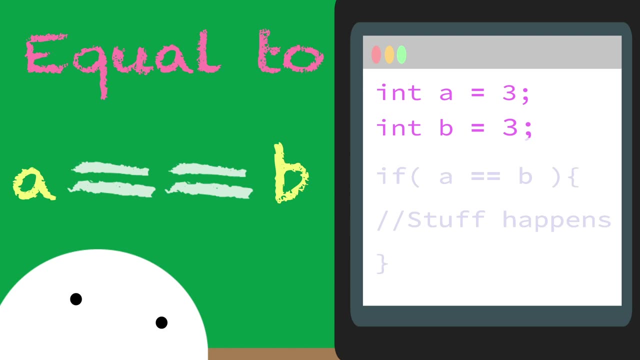 And in programming we write these symbols a little differently. Notice how equals to has two equal signs. This is because only using one equal sign means you're assigning values to a variable. So here we're saying a is equal to 3 and b is equal to 3.. 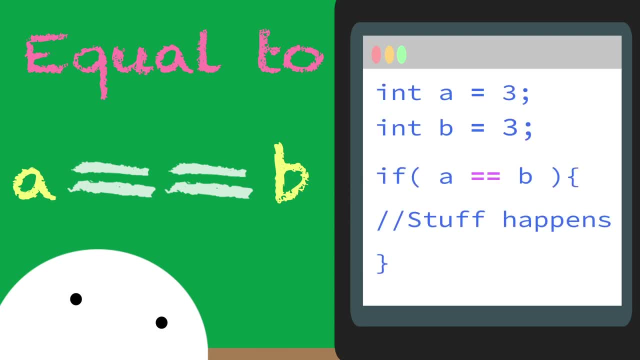 But when you use two equal signs you're checking to see if the left side is equal to the right side And if you want to check that something is not equal to something else, an exclamation point is a universal way in programming to represent the word, not So putting. 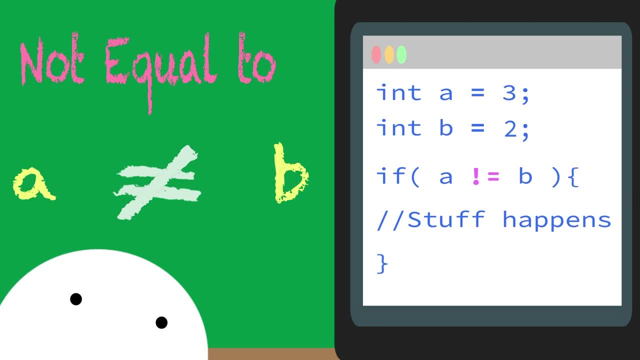 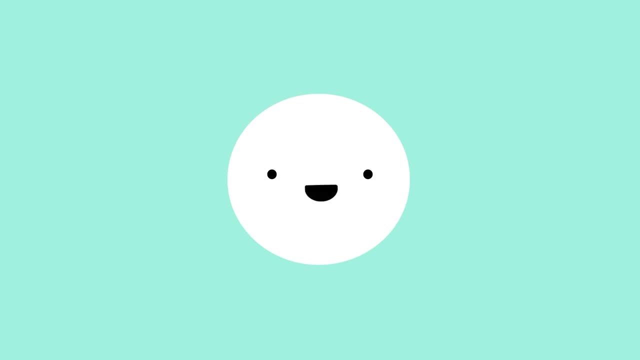 an exclamation point in front of an equal sign means not equal to. Technically the exclamation point itself is kind of another operator, but we'll get to that in a moment. So now that we know how, if statements and conditions work, we can look at an example now. 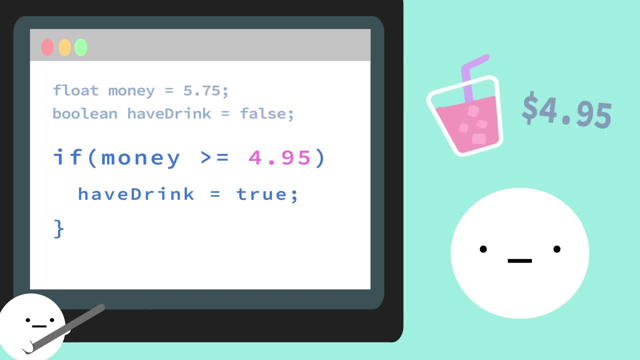 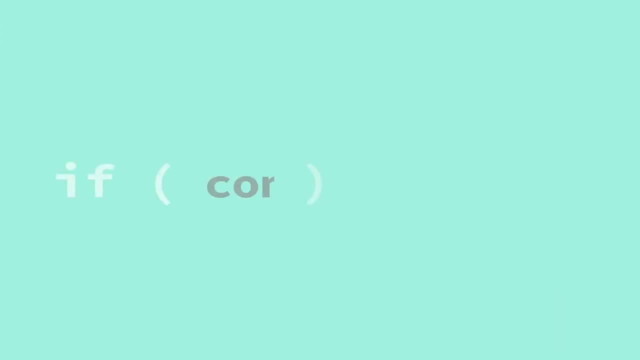 So let's say a drink costs $4.95.. I currently have $5.75, and I currently don't have a drink. But going into our conditional, since the money I do have is more than $4.95,, now I can have a drink. But let's say you want to check for two conditions in the same if statement. 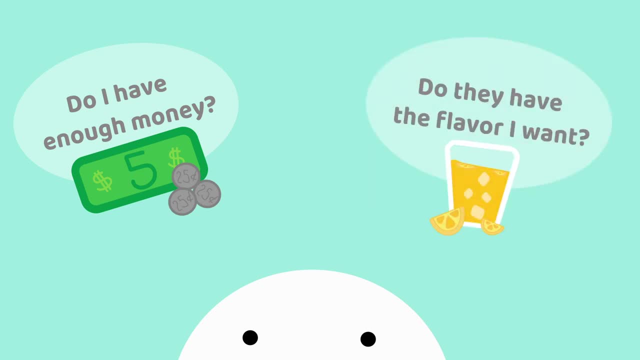 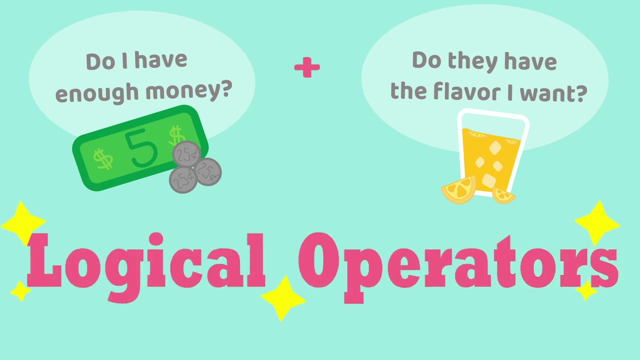 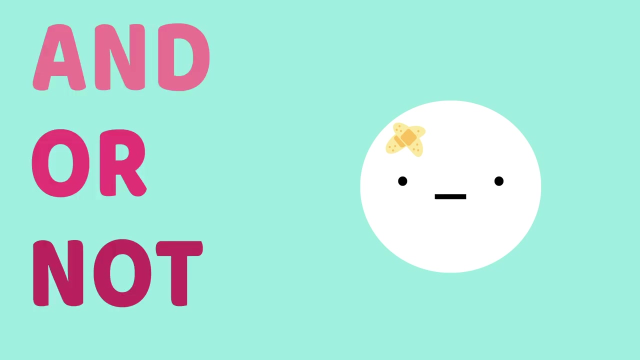 like: do I have enough money and do they have the flavor I want? In that case, you can combine conditions with what's known as a logical operator. Logical operators are simply the words and or and not. The nice thing is they work exactly how you would expect them to. in plain, 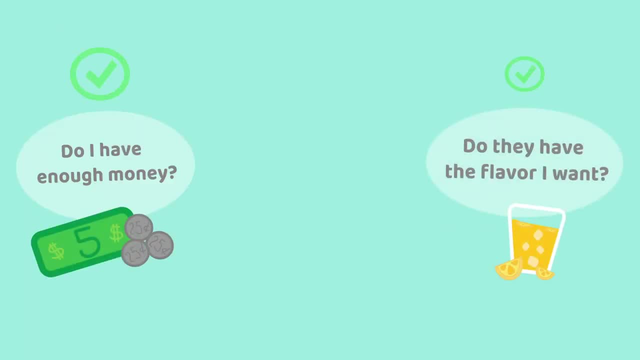 English. So if I want to check if two conditions are both true, we would use the word and, Which is represented by two ampersands. You know those little squiggly boys. So looking at this example, I want to check if I have more than $4.95,. 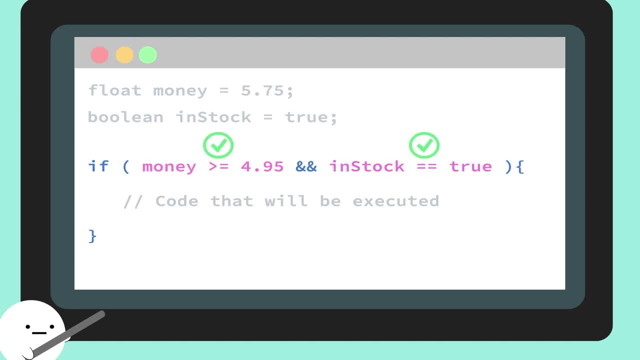 and that my favorite flavor is in stock. Since they are both true, the computer will run the code inside the if statement. But let's say we only have $3.50.. $3.50 is less than $4.95, which makes this condition false, Even though they have the drink we want and requires both. 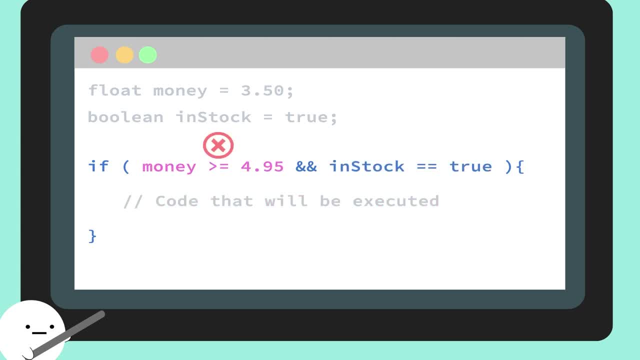 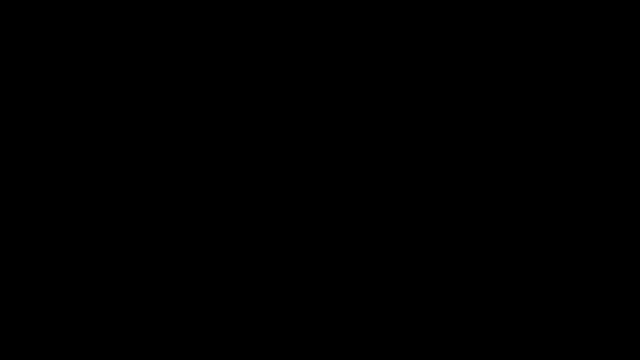 to be true to run the code. So since we have one condition that failed, the computer will ignore what's inside of our if statement and continue on with our program. If we want to check to see if at least one of the conditions is true, we would use the or operator Which. 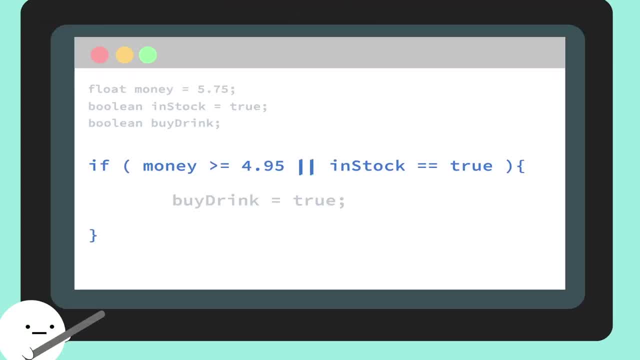 is represented by two straight lines. So if I have more than $4.95, or the cafe has the flavor I want in stock, I'll buy a drink. So only one condition needs to be true to execute the code, And if both fail, then the computer ignores the stuff inside and continues on with your program. 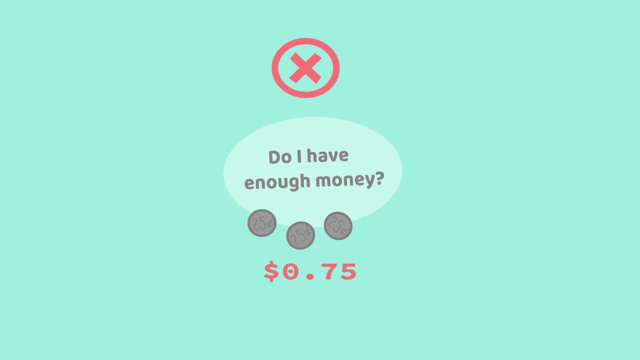 And, lastly, we can check if our condition is not true by using the not operator. As we mentioned earlier, the exclamation point is the universal way of representing the word not, So if we put the exclamation point in front of the condition, 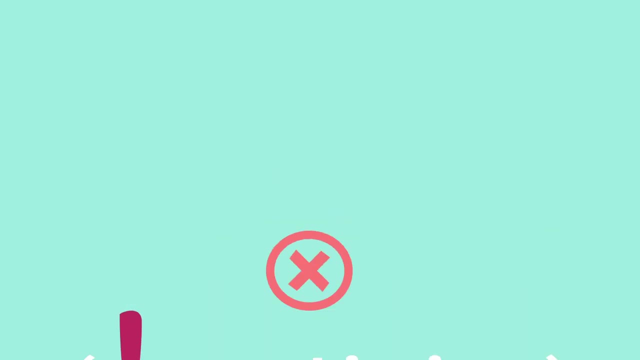 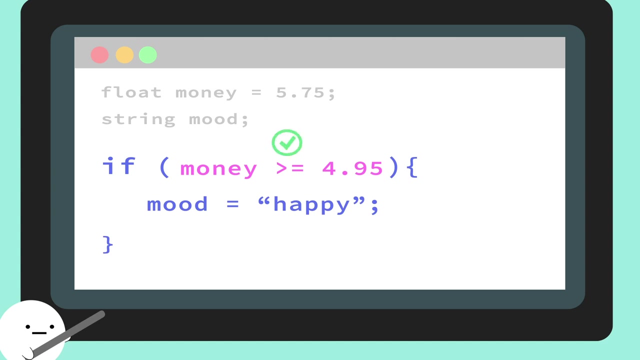 we can check that if our condition is not true. So we know that if statements check if our conditions are true, Without the exclamation point, our if statement would check to see if our money is greater than or equal to $4.95, then do whatever's inside the 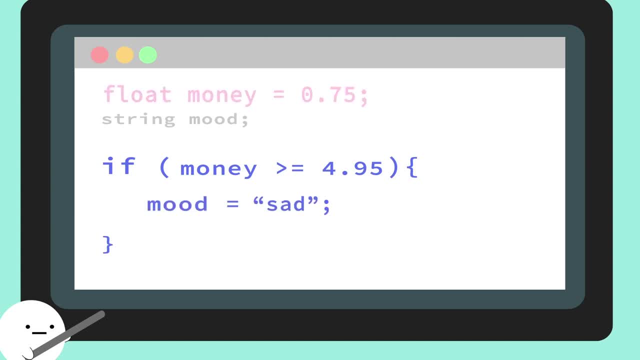 curly braces. But let's say I only have $0.75, and I want something to happen if I don't have enough money. If we put an exclamation point now, the if statement can check to see if our condition is not true and then proceed to the code inside the curly braces. So in this case, 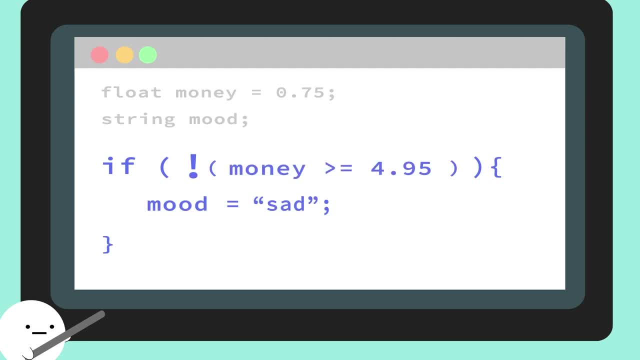 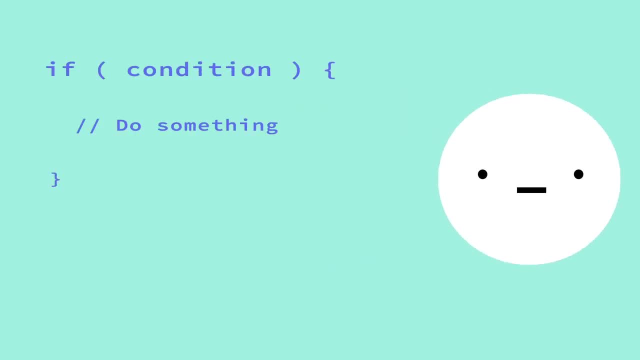 if we don't have enough money, then our mood is set to sad. Anyway, that's it when it comes to if statements by themselves Just check to see if something is true, Then if it is, it'll execute some code. 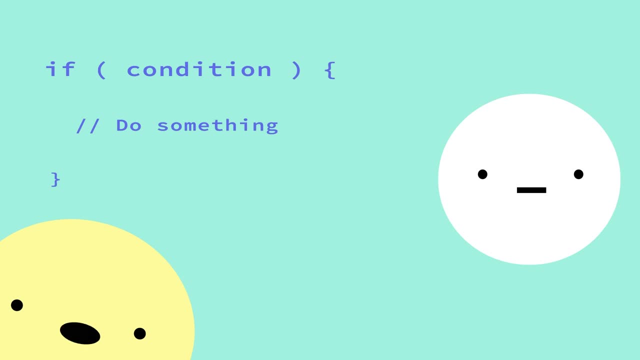 But uh, what if you want something to happen if your if statement fails? Well, I'm glad you asked Kevin, You would handle this with what's called an else statement. You attach this to the end of your if statement as a default action. 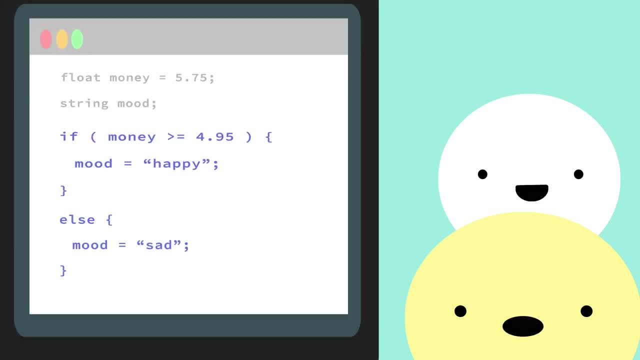 if your condition doesn't pass, Take a look. So if we have more than $4.95, then our mood is happy, Else we'll be sad. But let's say you have a few different decisions to make, Like for example: 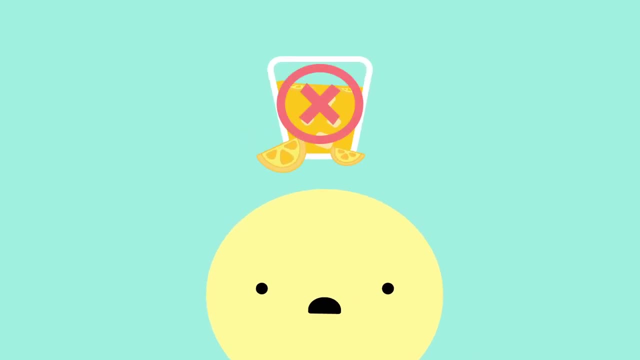 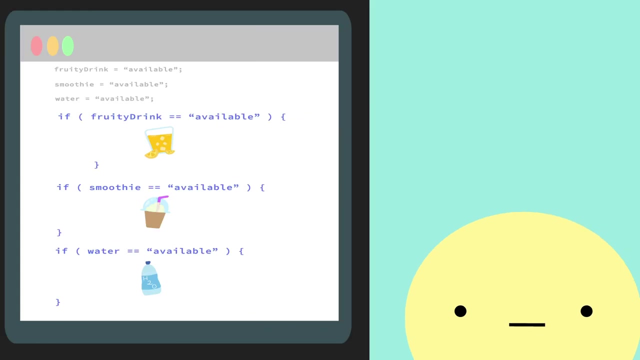 Kevin here wants something fruity if it's available, But if it's not, then he'll get a smoothie, And if they're out of that too, he'll just get a water. Well, if we write this with three different if statements, look what happens. 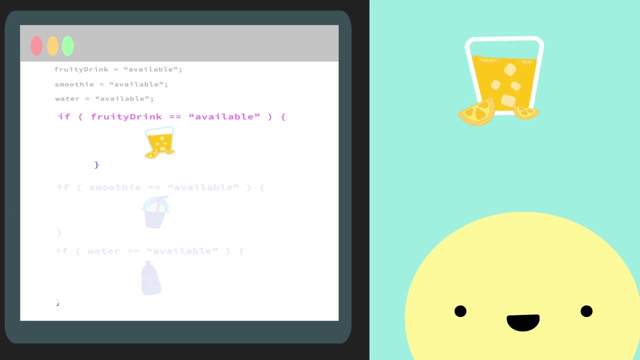 Fruity is available, so great, we can get that. But now our code continues, and now we've also bought a smoothie and we've also gotten a water. since they're all available, Now we've got all these drinks that we want to drink, And now we've also bought a smoothie and we've also gotten a. 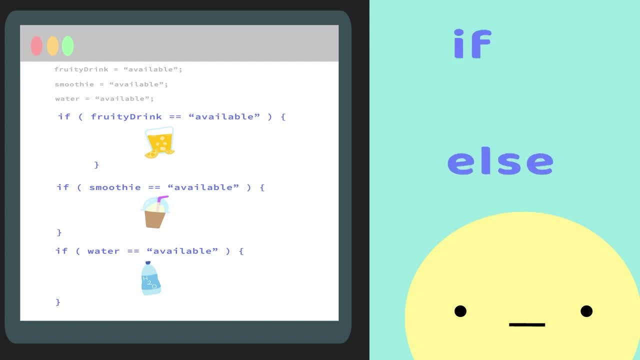 smoothie that we didn't want To avoid this. we can combine if and else statements to make something called an else- if statement. That way, if our first condition is met, in this case, we get something fruity, our code will stop there and we won't have to buy everything else. 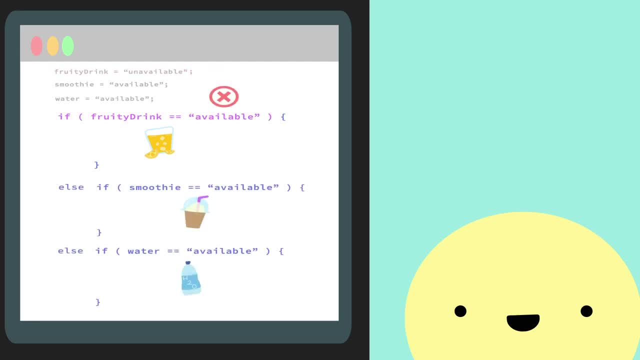 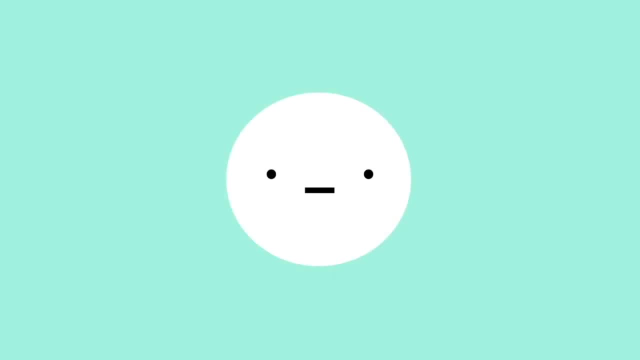 But if our condition doesn't succeed, then it'll continue down the rest of the else if statements until one of them passes. So that's if statements in a nutshell. Now let's put all of this information together with a couple of examples. So let's put all of this information together with a couple of examples. So that's if statements in a nutshell. Now let's put all of this information together with a couple of examples. 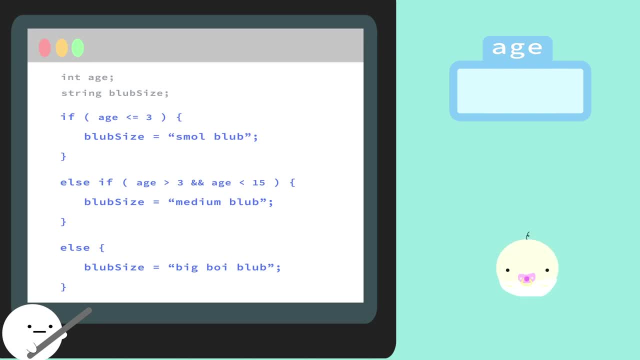 So that's if statements in a nutshell. Now let's put all of this information together with a couple of examples. So this is Blub Jr. As Blubs get older, they get bigger, So we can give them size categories based on their age. Here, Blub Jr's age is 3.. 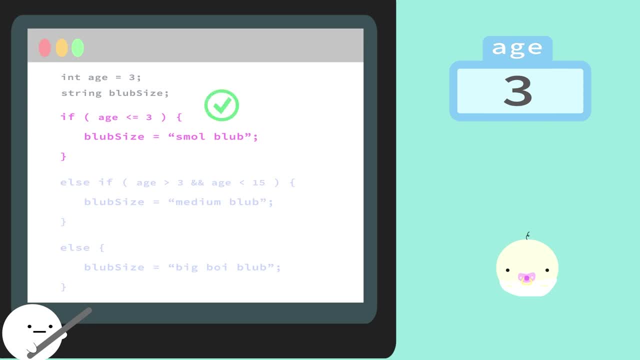 So looking at our first if statement, we see that if his age is less than or equal to 3, he'll be classified as a small Blub and the program will skip the other two conditions. But let's say he gets older and his age is now set to 12.. 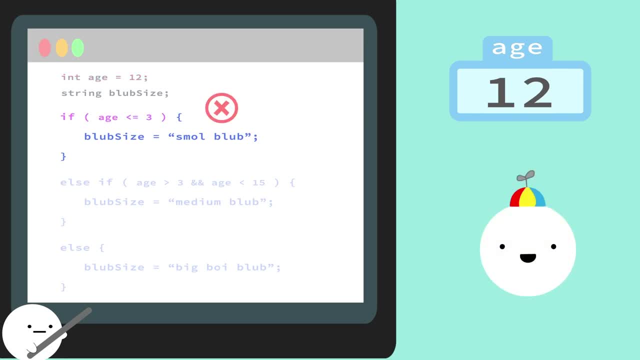 Since 12 is greater than 3, our first condition will fail and our program will move on to the second condition. Now, since Blub's age is between 3 and 15, our condition here will pass and now Blub is classified as a medium Blub And finally let's say Blub is all grown up at. 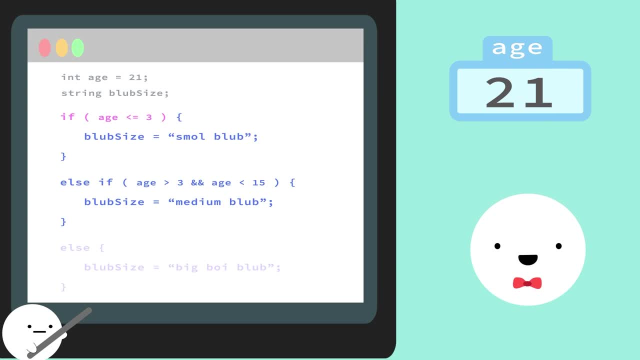 the age of 21.. Since 21 is greater than 3, our program will skip the first condition and move on to condition 2.. Looking at our condition here, we see that even though 21 is greater than 3, it's not less than 15.. And since our AND operator requires both conditions to be true, 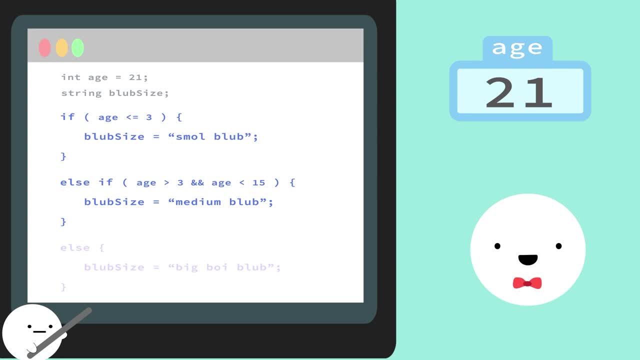 this condition will fail as well. Since neither of these conditions pass, we're left with our else statement, which will let us take care of any other age that isn't handled by the other two conditions, making this Blub a big boy. Now here's a more complex example with an 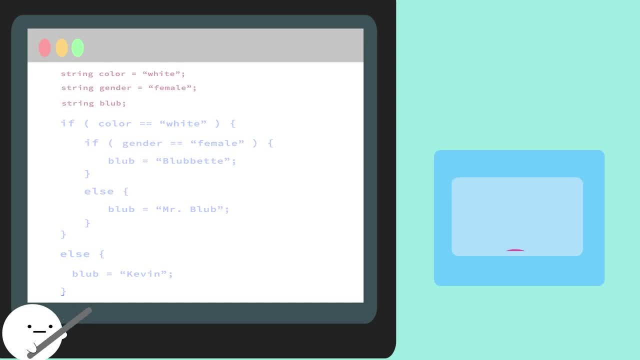 if statement inside of an if statement. We want to identify our mysterious Blub. We first check if our color is white. It is, So we go inside our curly braces. but now we see there's another if statement nested inside our other one. 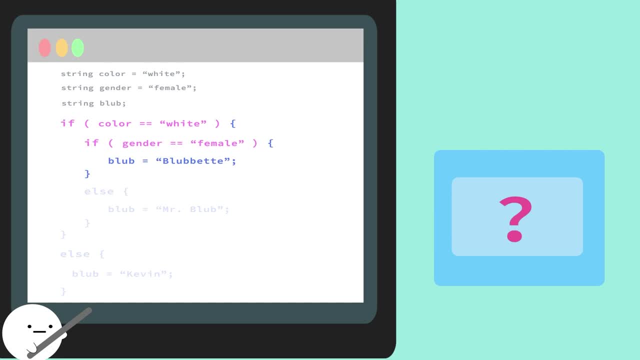 Nested. if statements help us get more specific with checking our data, In this case we can get more specific information about our mysterious Blub. If they're a white female Blub, then this Blub is identified as Blubette, But if they're not, then it's identified as Mr Blub. 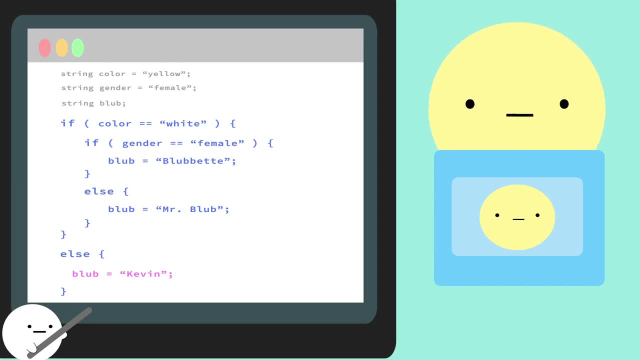 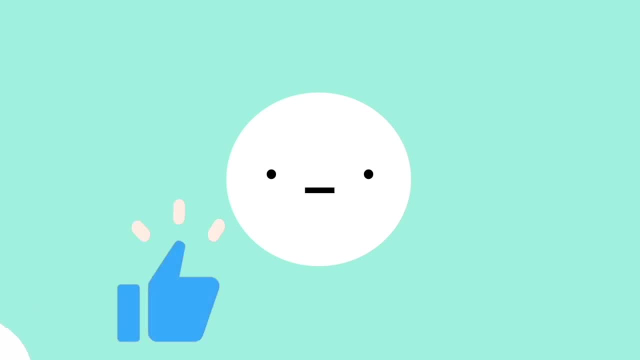 And if our mysterious Blub isn't even white, then they're probably Kevin. That's it for today's video. We hope you've learned something and if you liked this video, please like, subscribe and hit that notification bell so you'll know when. 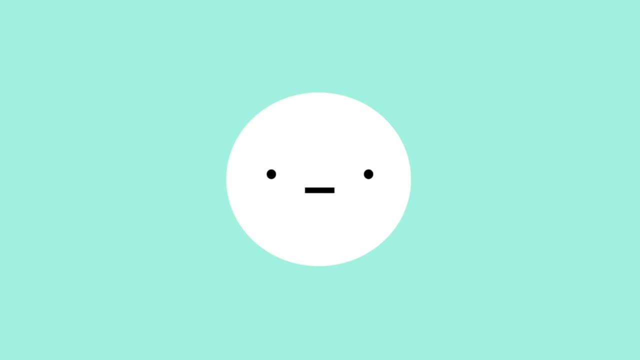 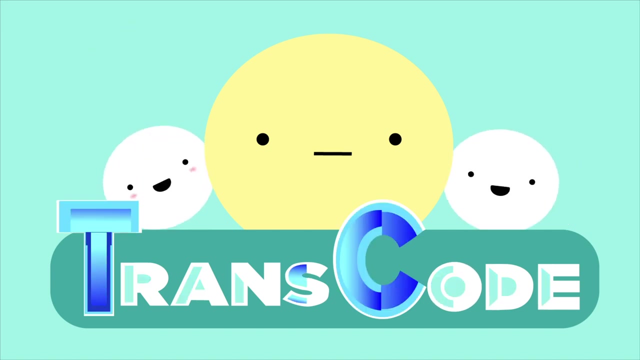 our next video comes out. Also, let us know of any topics that you would like us to cover next time, And we'll see you again in the next one. Say bye, Kevin, Bye, Bye.